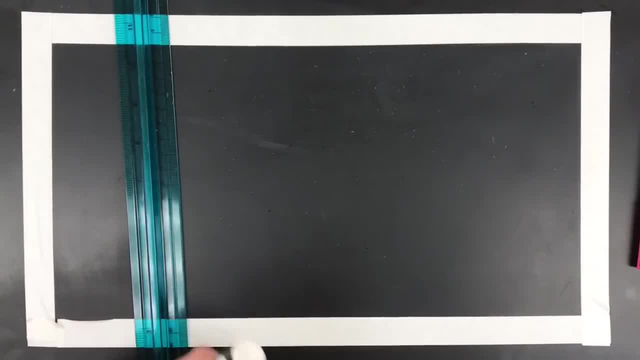 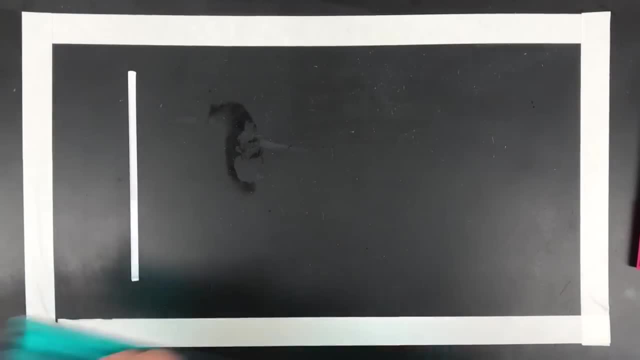 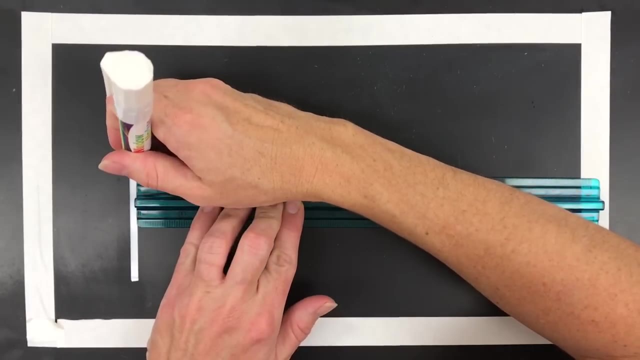 the labeling first. So I'm going to draw the two axes for these waves, and you'll use waves in chemistry and you'll use waves in physics and sometimes in mathematics. you will also draw a sine or cosine waves too. So we're going to draw these two axes For science. this is going to be. 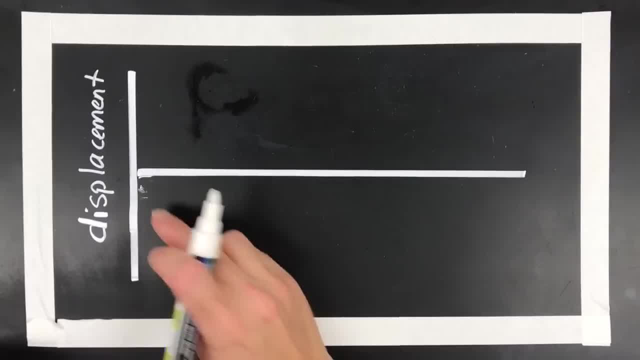 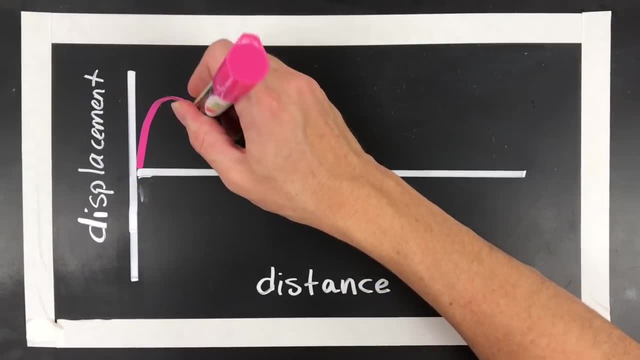 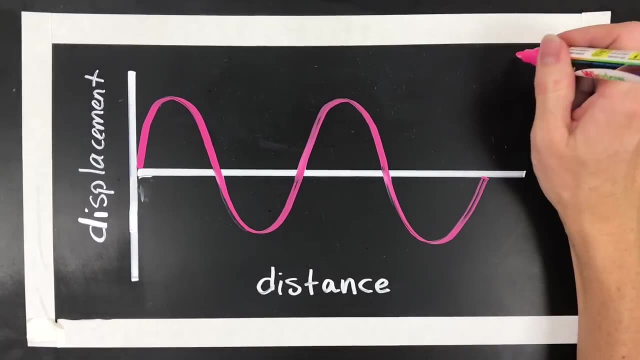 called the displacement. This direction is going to be called distance. Next I'm going to do is just give it a shot and draw a wave. So I'm going to go up, back down, hit that point again and try to make it look the same, and back up, And let's say that that took one second, you know, to happen. 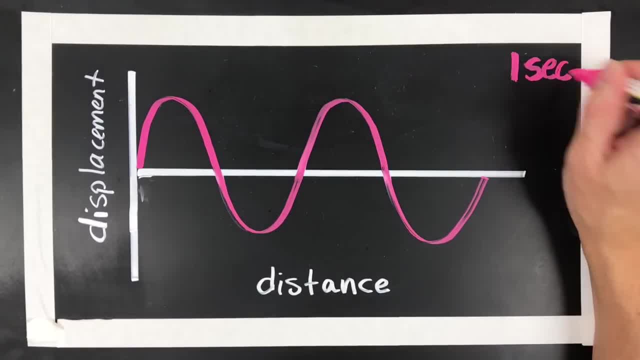 Okay, that's going to help us with frequency, So one second. So let's label all the components. The top is the crest You actually have. we have two crests here there, and there Down at the bottom is called the trough. So here and here. 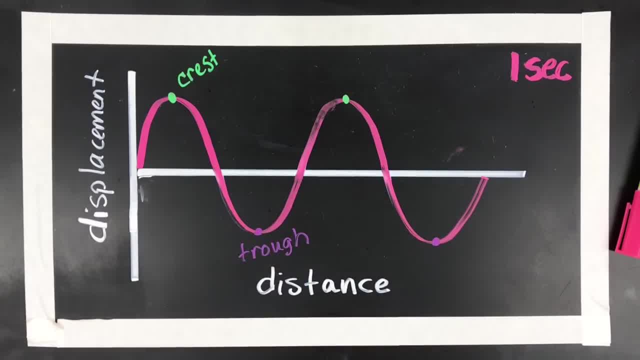 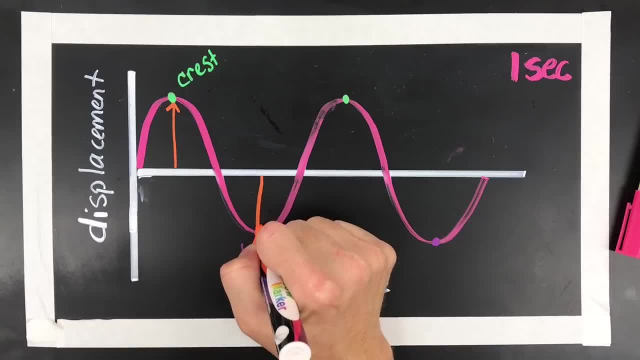 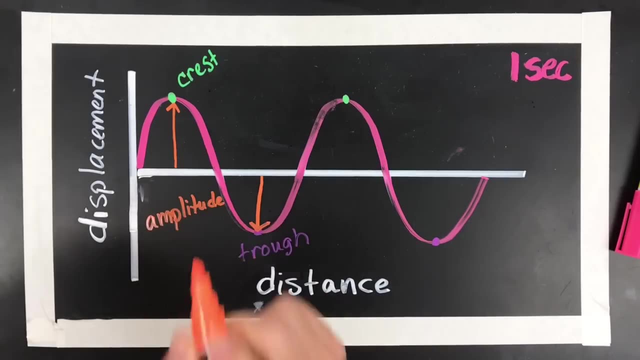 are called trough. Amplitude is actually from here to here, you know, and really, amplitude it can go downwards too. Okay, so that's amplitude. And then the next thing would be wavelength. There's a couple of ways to do wavelength. You can do. 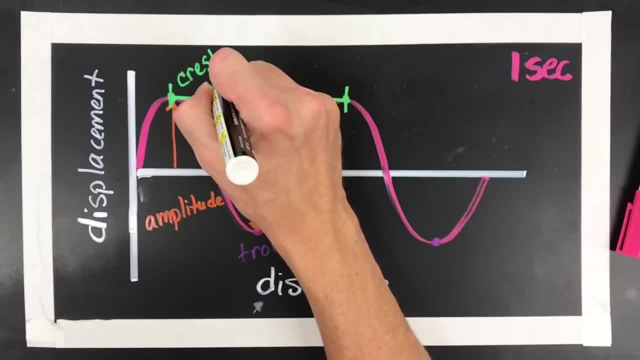 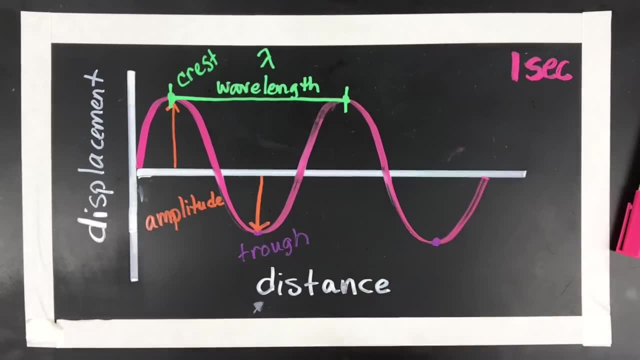 crest to crest, here to here is wavelength. Don't get confused. A wavelength is given the symbol lambda, So you might see that some people will label trough to trough as wavelength. But to be honest with you, there's one more thing that's important. This line is called the resting. 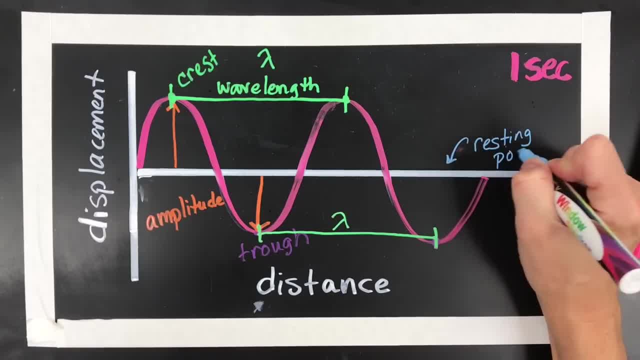 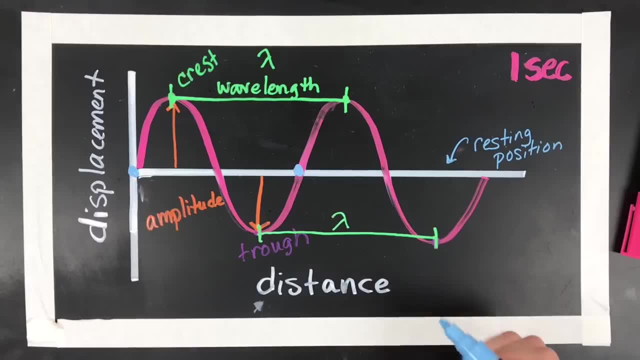 position And you can do, you know, kind of what I call resting point to resting point. So, for example, we started here and the wave ended there. That is also wavelength. From here to here is also wavelength. Okay, not a very good lambda there, but there we go. The last thing would be frequency. 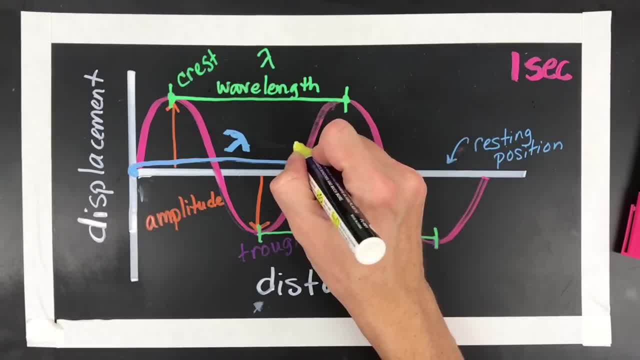 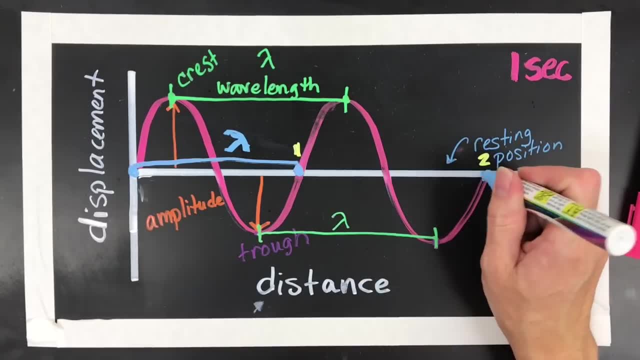 So frequency is the fact that I had one and then I had this wave go up and back down to a. you know, the resting point came again here. So it started, it went up and down and then it landed there. So I have a frequency of two. 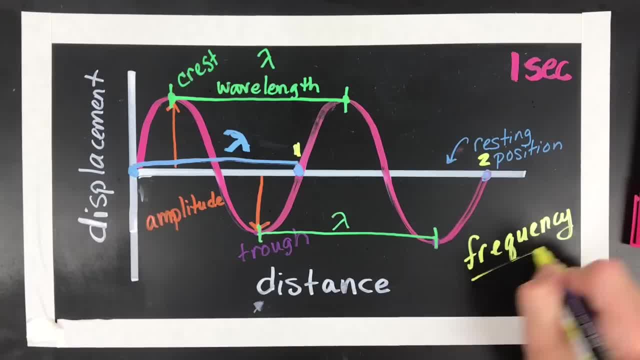 So frequency is just how many cycles happen per second. So I would say I had you know a frequency of two in this one second of time. Alright, we're gonna move on to the next part of the video, which is how to graph these waves. 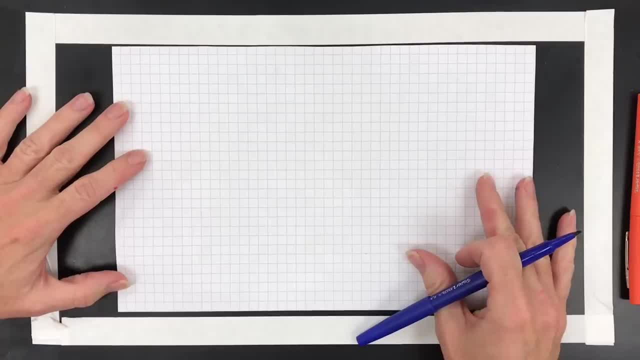 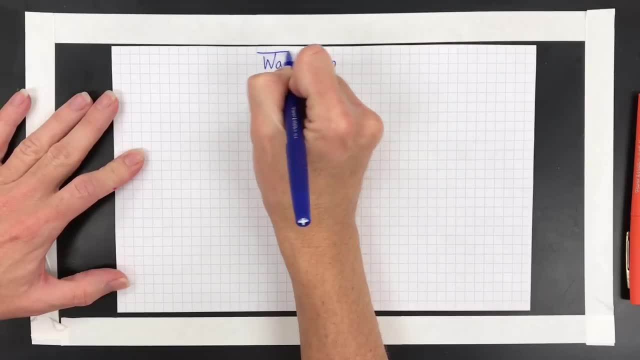 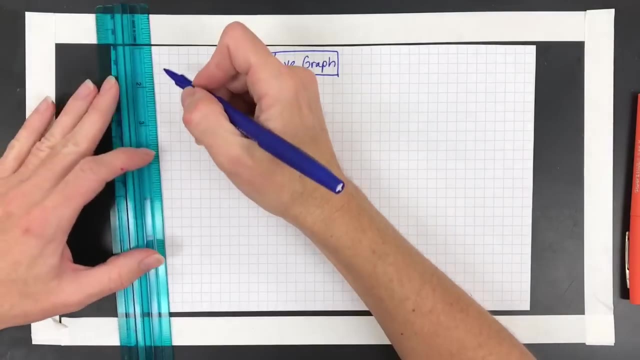 So the first thing you're gonna want to do is have your graph paper and put a title on it. I'm just gonna title mine wave graph. You'd probably put a better title on it if you were doing physics or chemistry or mathematics, mathematics. but we'll just call it wave graph. Then the next thing is to draw your axes here. 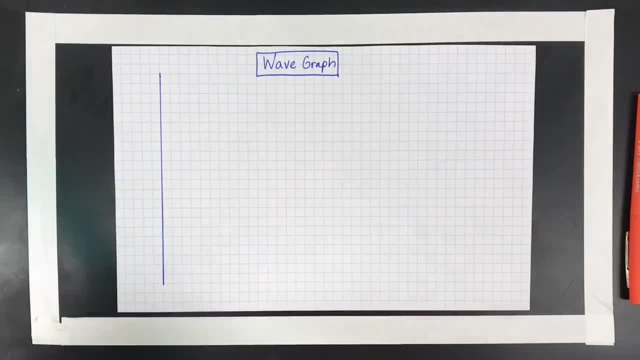 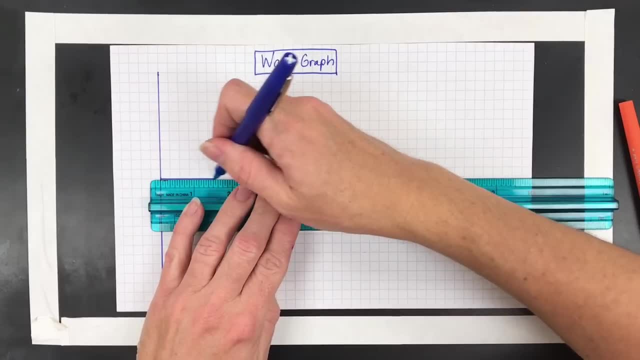 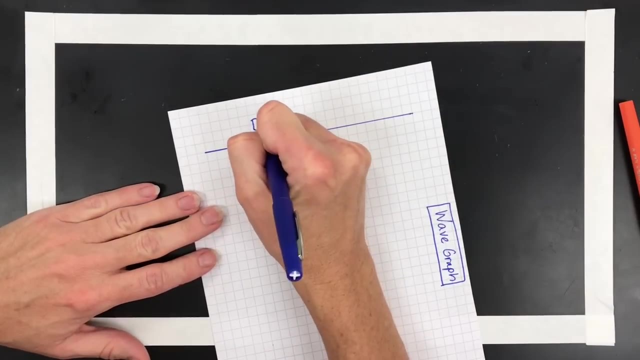 Use a ruler, get a nice straight line, All right, And then we'll find that middle point which is about here, And that's going to be called our resting position for a wave graph, Okay, And then displacement, or really this is going to be amplitude, but let me just call it. 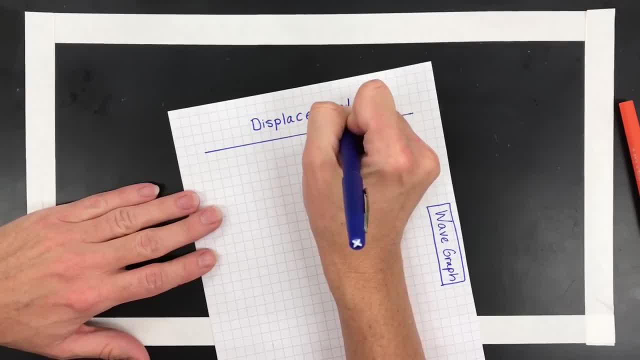 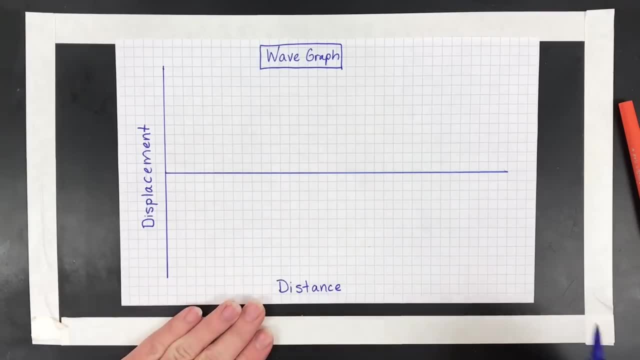 displacement. That's kind of a nice catch-all label that works for most subjects. And then down here, the most common label for physics and chemistry is going to be distance, And then I'm just going to say that this happens all in one second. Okay, I'm just going to pick some arbitrary 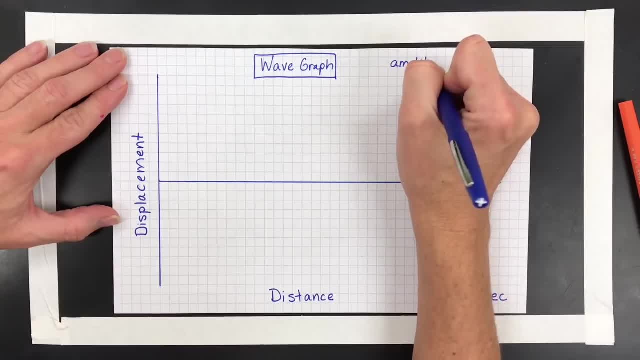 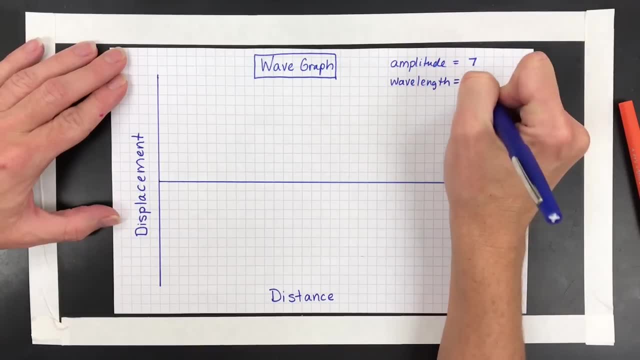 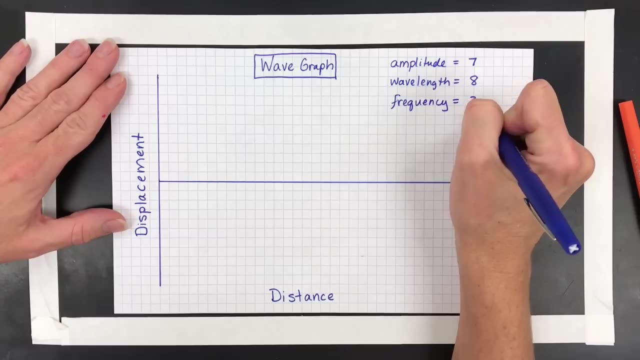 numbers. I'm going to make my amplitude seven. I'm going to make the wavelength eight- Nice even number, That'll help us graph it easier. And then let's just make it a frequency of three. That means I'm going to have three. 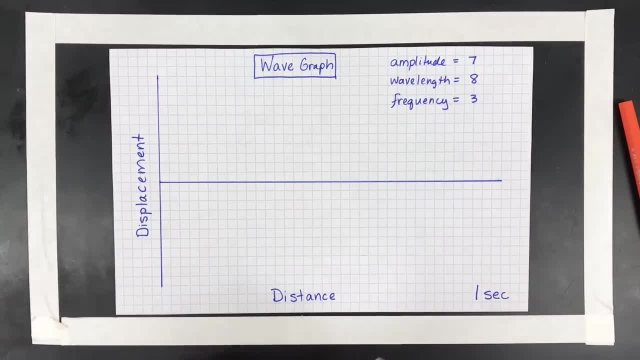 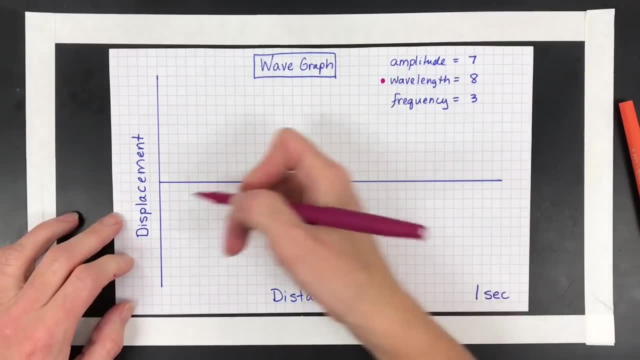 cycles of this wave in one second. Okay, So I'm going to switch colors. I'll try to do a color for each, each one of these. So wavelength- I'm going to start with wavelength. I'm going to do like a kind of a pinky color here, So you're going to end up needing a wavelength of eight. 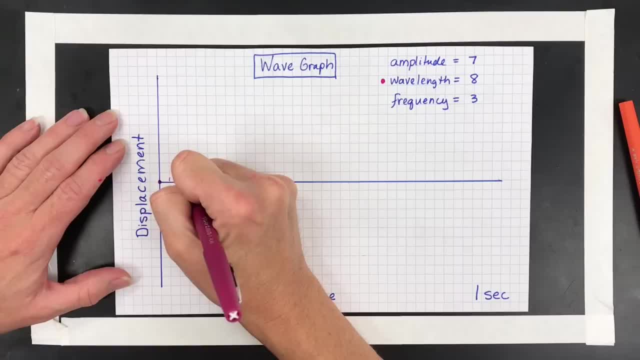 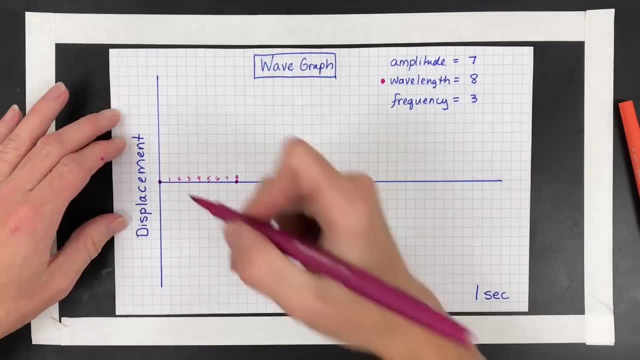 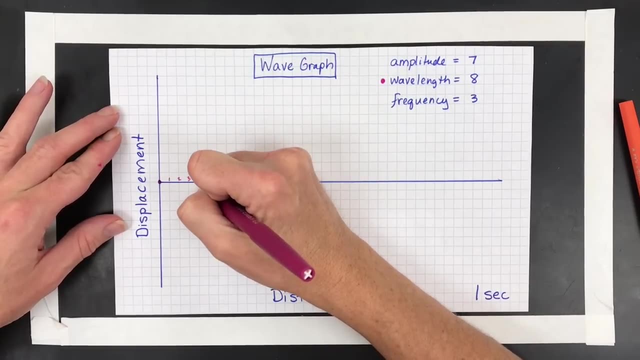 So I'm going to start at zero and then one, two, three, four, five, six, seven and eight. So that is going to be where my wave is going to crest: go through the resting point down to the trough and back to this resting point. Halfway through it's going to cross this resting position. 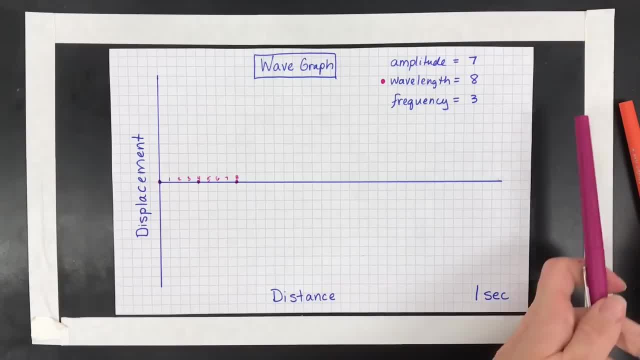 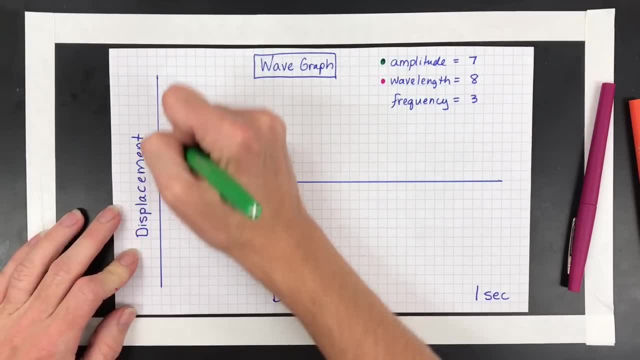 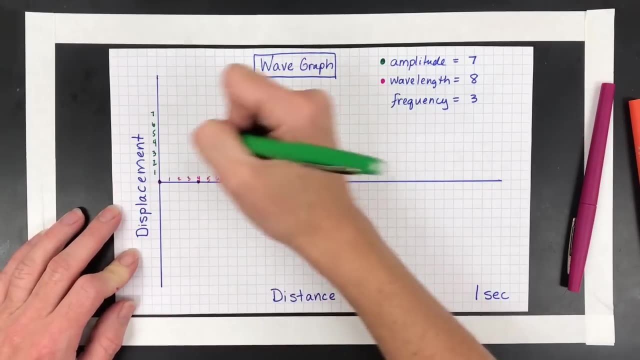 line, And then those are kind of the key points for wavelength. Next thing we're going to need to do is amplitude. Amplitude I'll do in green That's going to be how far this wave goes up and down on this graph. So one, two, three, four, five, six, seven is going to be the height. 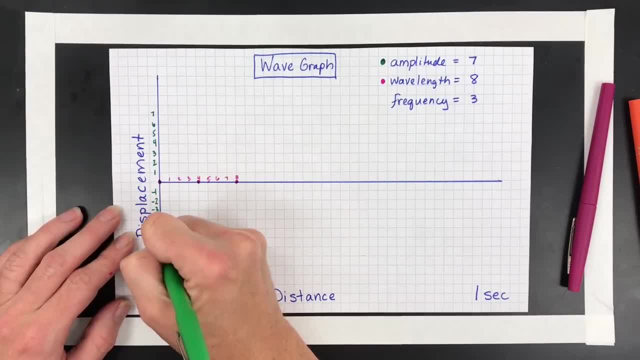 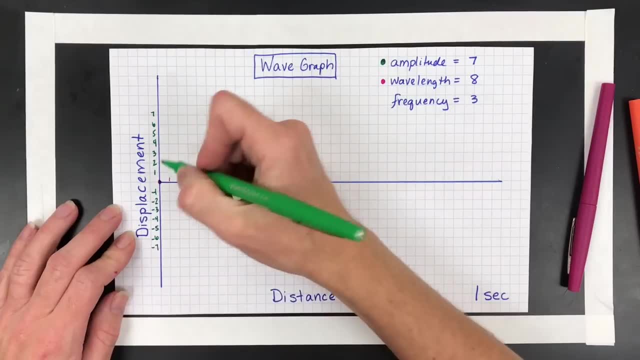 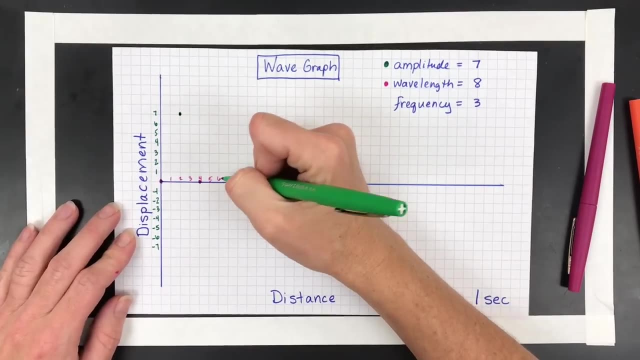 And then same for going down. I'm just going to put negative numbers just to symbolize that I'm going in the downward direction. there, Halfway between the zero and the four, is where our crest is going to be up at seven. So I'm going to go to two and then up to seven. Same thing here. 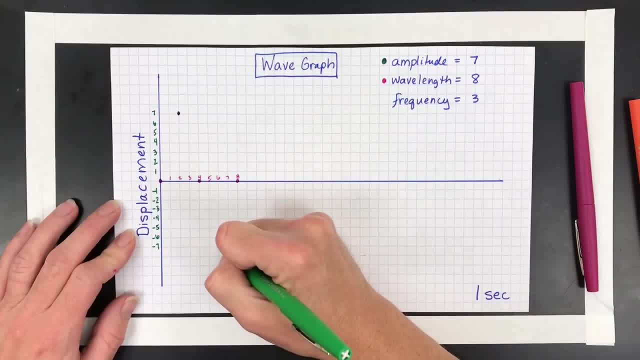 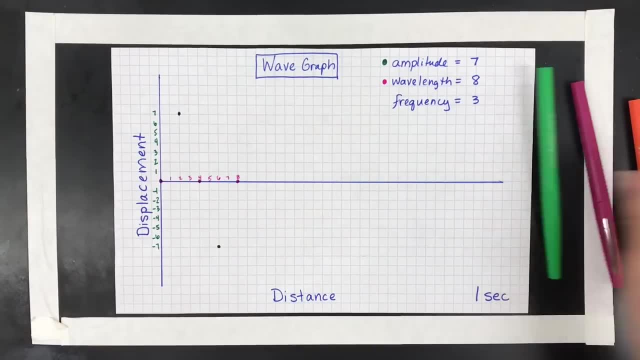 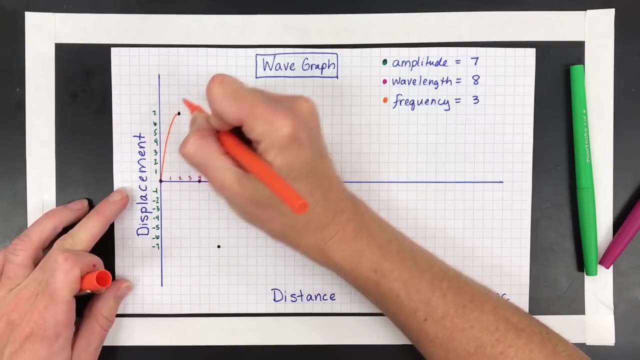 halfway between four and eight. you're going to go down to seven. So six is the halfway point between four and eight and go down, And then what we want to do is- you know, I'm going to do orange for frequency- We want to make this be one cycle. Okay, Sometimes it's called a period. 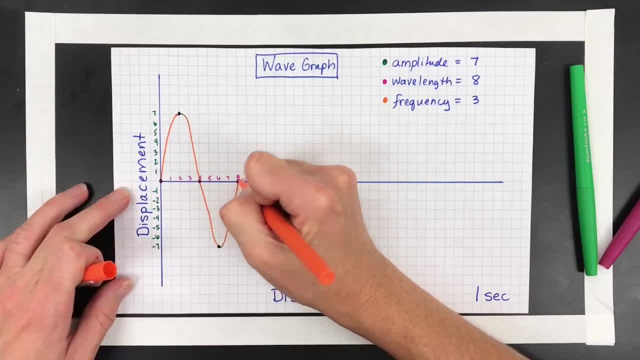 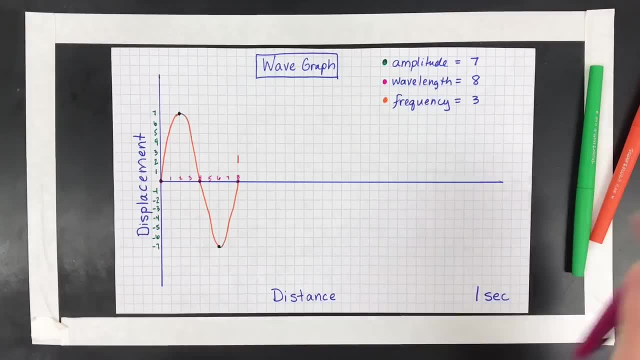 too, but we'll just call it a cycle, make it easy. So there's one. Okay, So that would be a frequency of one in this one second, but it's a frequency of three. So what I need to do is I need to graph. 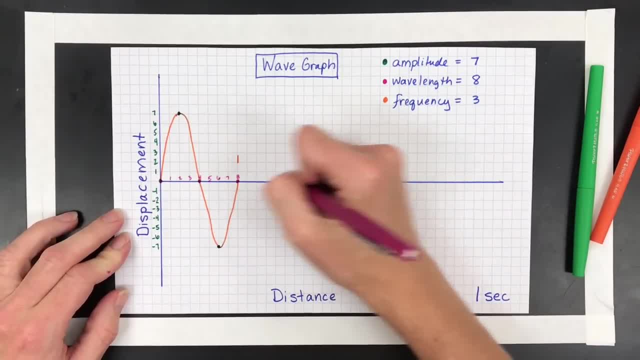 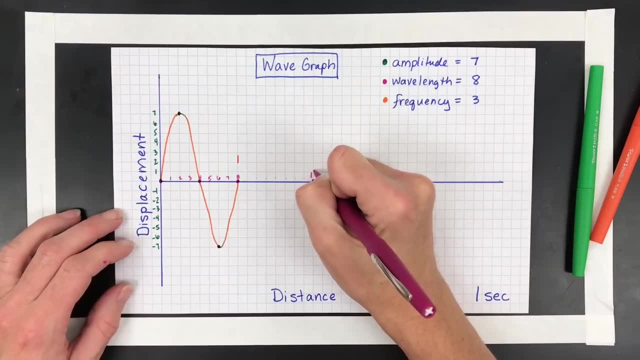 this two more times. So I'm going to go out eight more. So nine, 10,, 11,, 12,, 13,, 14,, 15,, 16 is here, So that's going to be our next wave. Halfway will be right there, And then I'm going to switch. 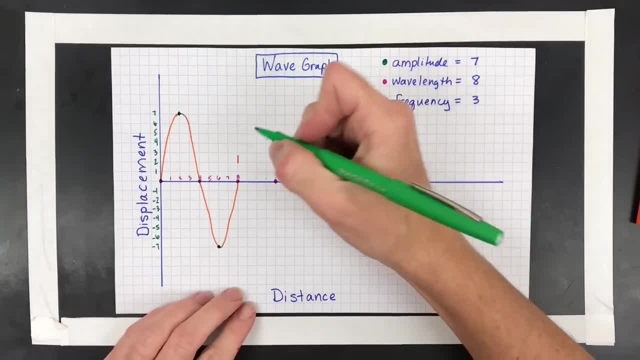 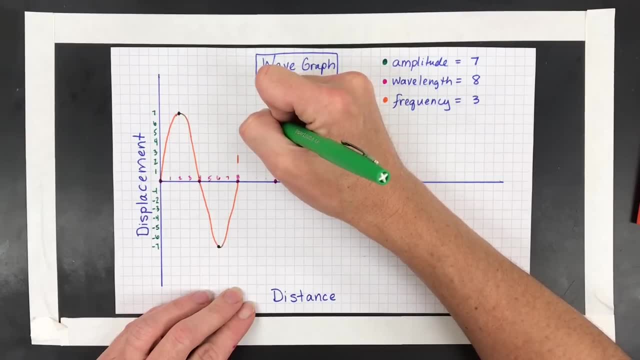 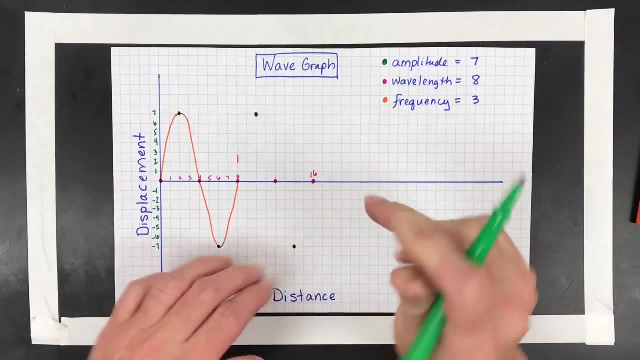 colors. Amplitude is again the height of the crest and the trough. So halfway between here is going to be, on, you know, nine and 10, and then up to seven. same thing. Halfway between here is going to be your 14 and then down to seven, And then to show that I did another cycle. 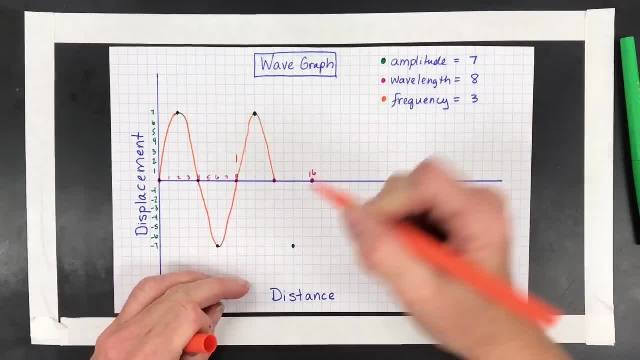 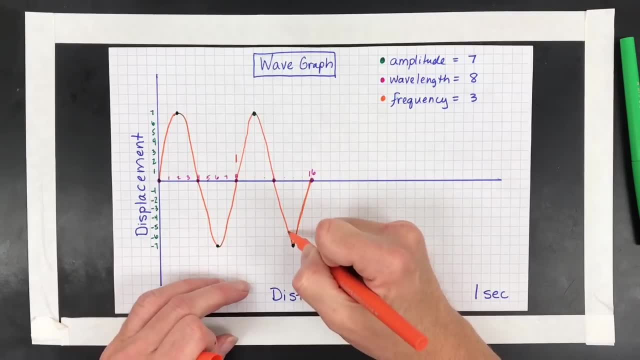 I'm going to have the wave go crest through the resting point back down to the trough and up to the uh resting point again. try to kind of smooth this out a little bit. That one was a little sharp, All right, One more time. 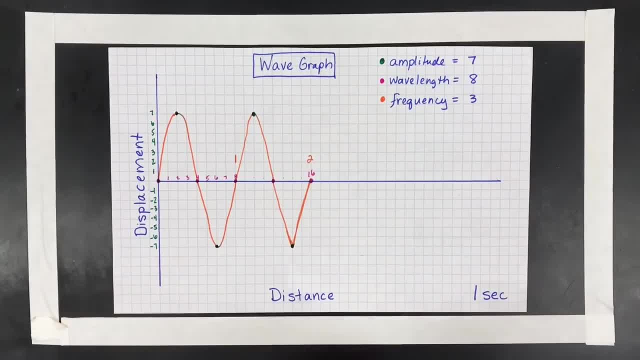 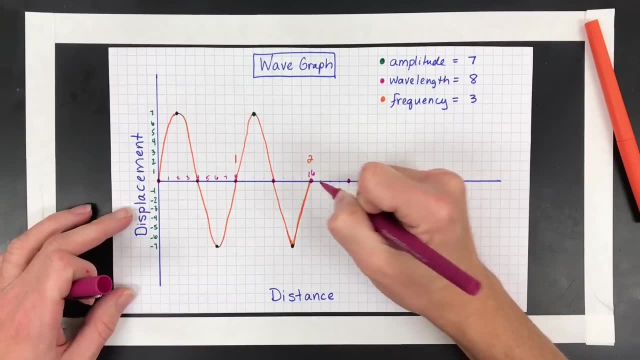 Cause. again, that's a frequency of two. So I needed a frequency of three. same thing: two, three, four, five, six, seven, eight, and then mark your halfway points. Those again are where your resting points will be. for your wavelength, You're going to have a crest and a trough. 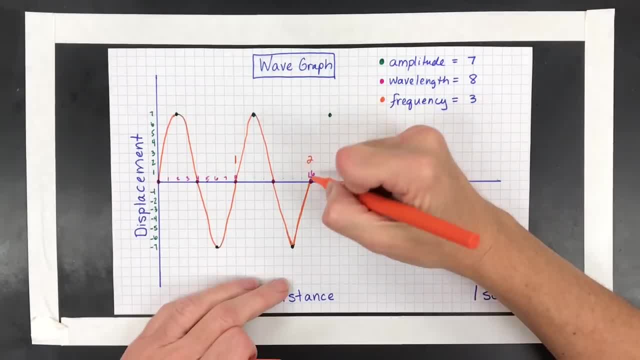 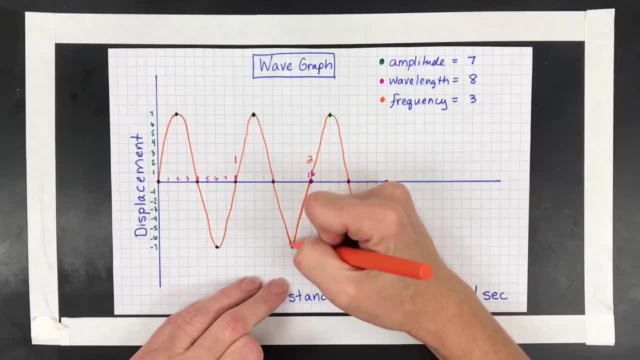 at those points and then draw again. I are nice, smooth, hopefully smooth- wave, trying to make it a little bit more smoother than the last time. There we go. So there's a little mistake there, but that's still fine. Okay. Now how does this relate to chemistry? So the big